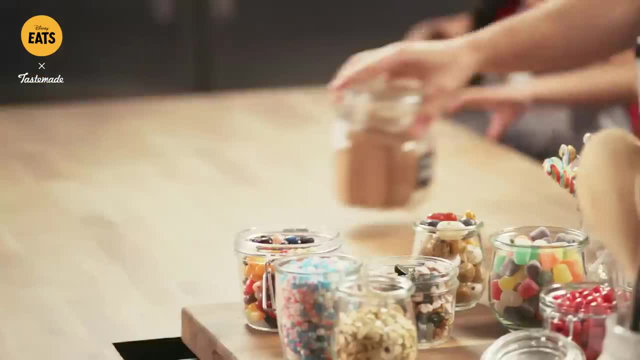 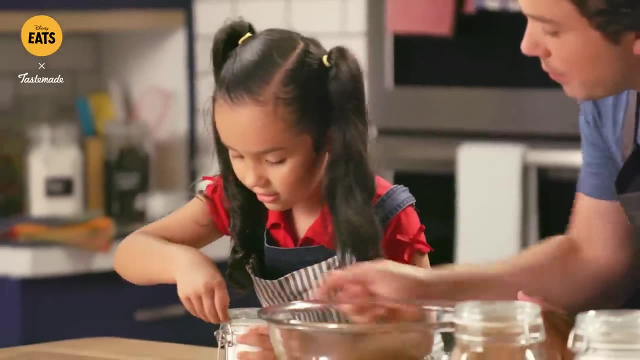 We'll need sugar and baking soda And then cocoa powder. OK, First we'll need to put in this Baking soda from the bottom. There it is OK, So hold on. No, That's a lot, Sammy. 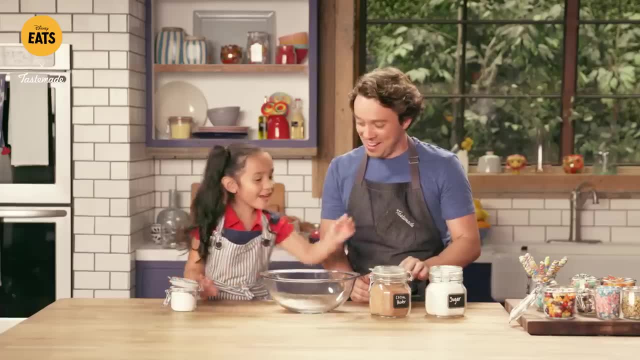 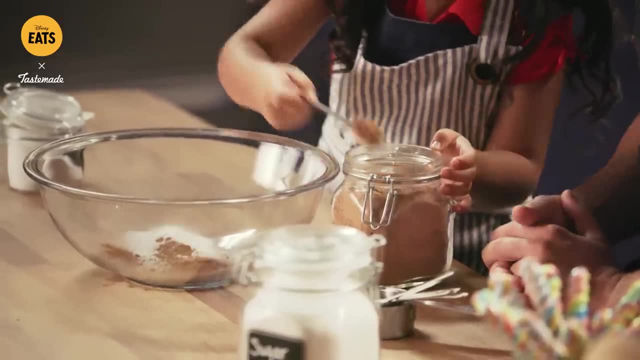 We need a lot. I think that's enough. Then I think we'll need over here, OK, Some cocoa powder. Let's see. Do you remember if there were any measurements? Man, you're the boss. I told you All right. 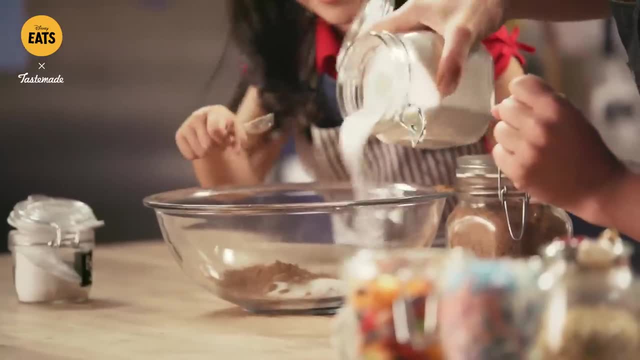 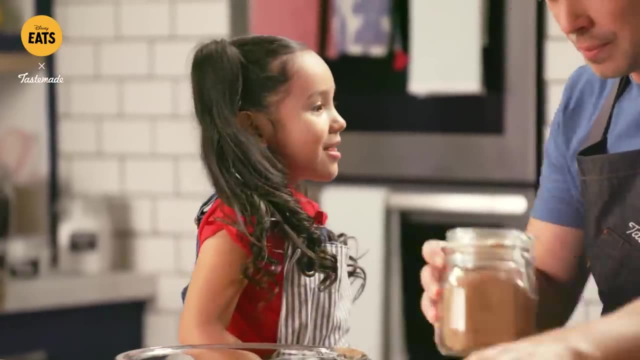 And some sugar. Yep, What do you think? OK, Put too much. You put a lot of baking powder. I got to balance it out somehow. Now do we have a mixer That's the kind We're going to take it and start stirring it. 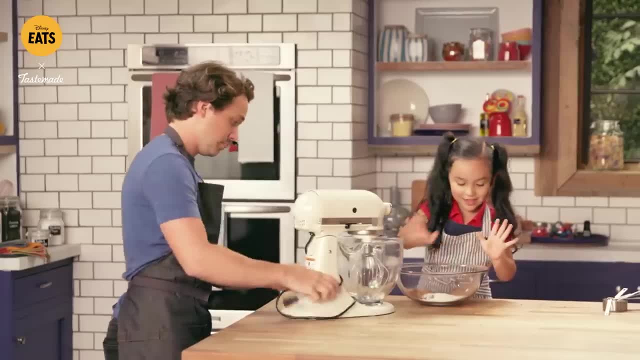 I mean this I can mix by hand. Is there something else that we're mixing? Let me go check. Hmm, Oh, berries and cream. That's great. There's mint in here, Sammy. Oh cool. Do you think we need mint? 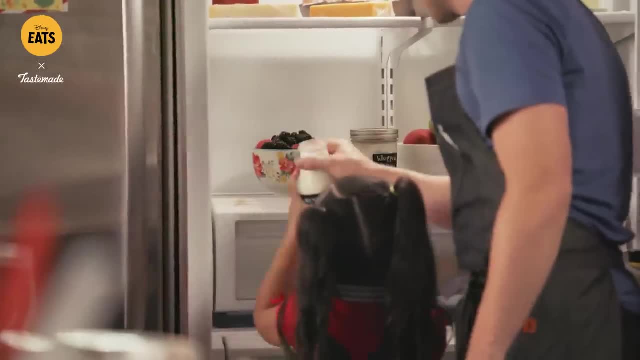 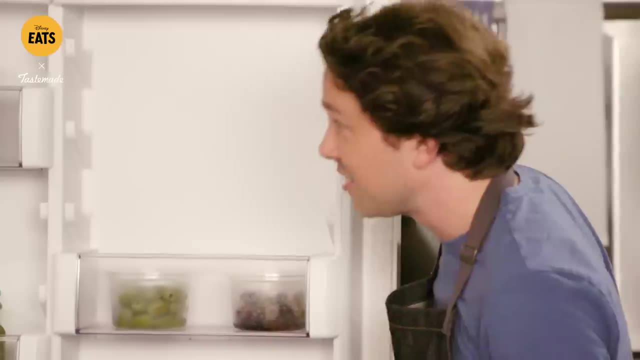 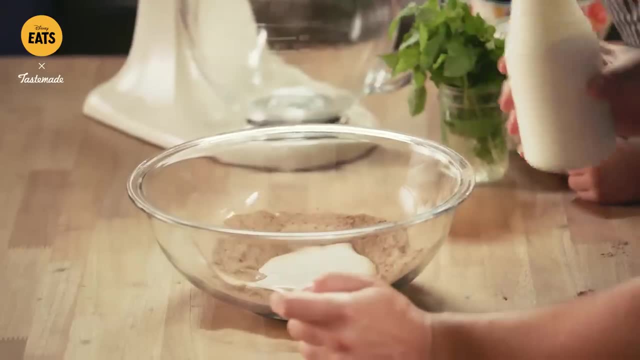 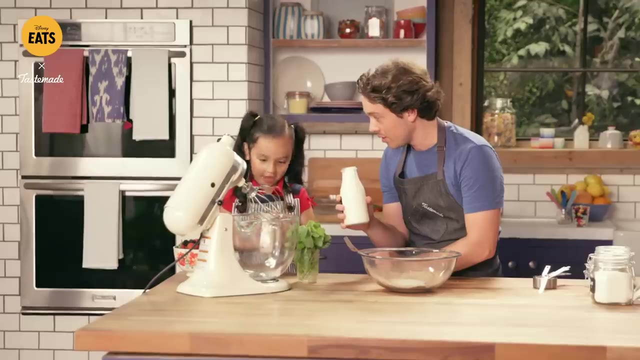 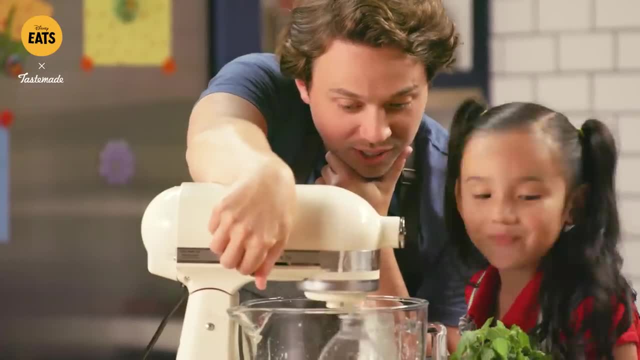 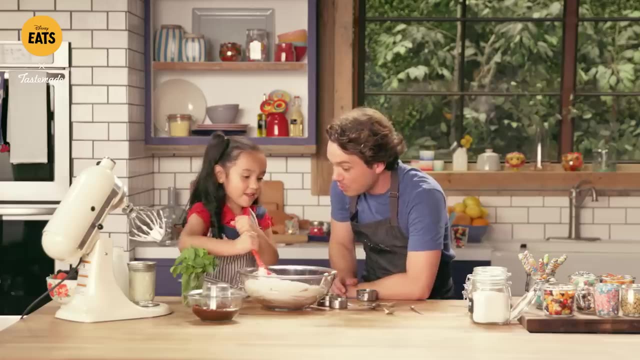 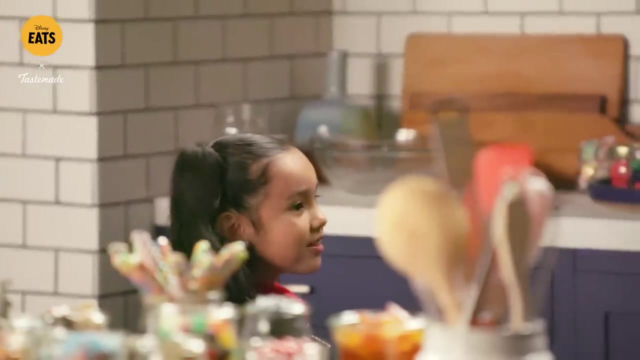 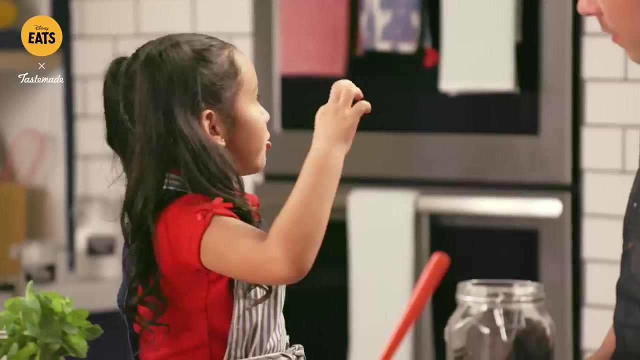 Mmm. Whipped cream Spatula. Mmm. What happens to whipped cream when you mix it too much? Nope, Sometimes it turns into butter. We don't want that to happen. Nope, Now we need cream cookies. how about these chocolate wafers? do we have a plastic bag here? why don't? 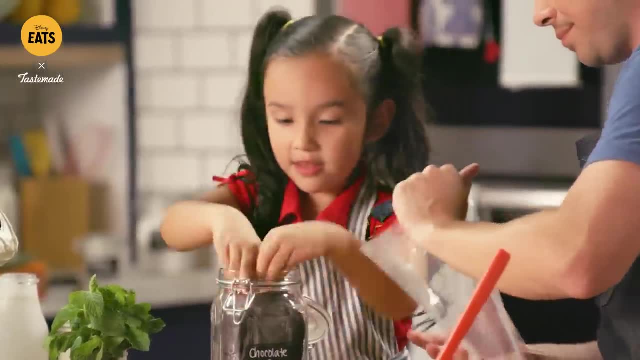 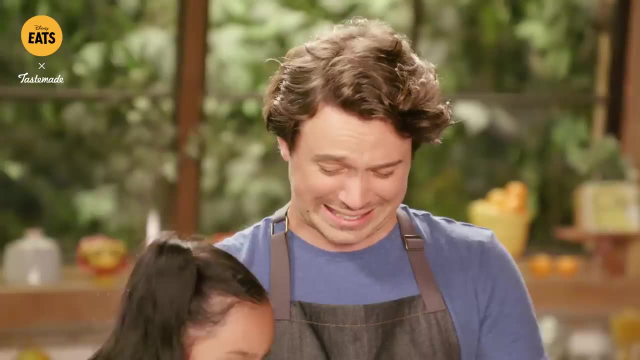 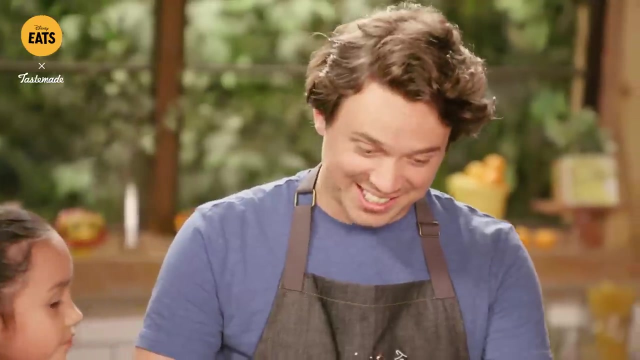 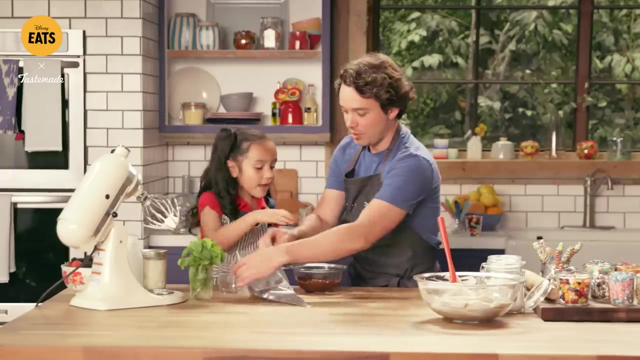 you reach in and put in some cookies, and then it's gonna crush up into big little pieces. can i give it a try? okay, that's great, thanks. okay, we're gonna grab the smushed ones and put it in until i say stop, okay, and then we're gonna grab the melted chocolate. 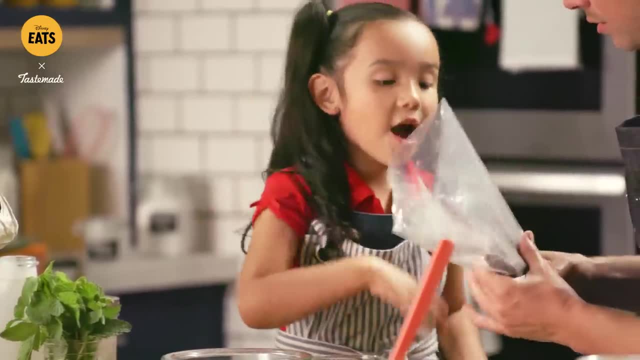 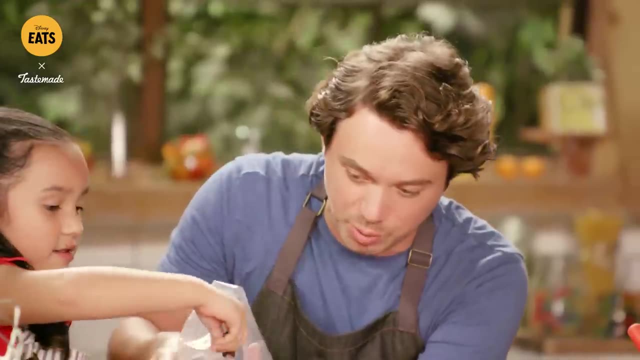 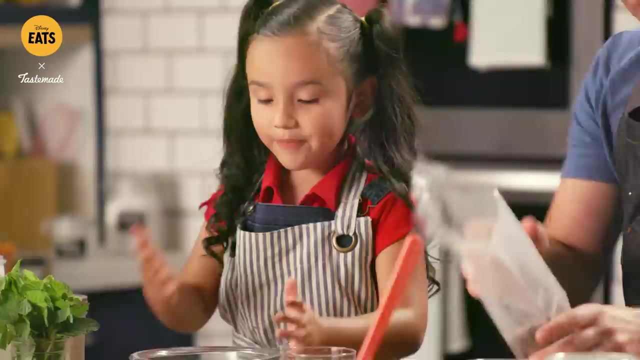 and pour a little bit until i say: stop, okay, then we're gonna do the same thing with this, then this, then this, then we're gonna do something special, okay. so here, let's pour a little in. we're grabbing it, okay, i'm putting it in. okay, stop, okay, stop. let me get a spoon so we can be, uh, we. 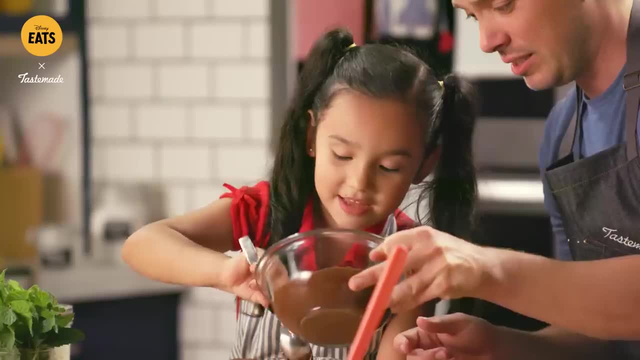 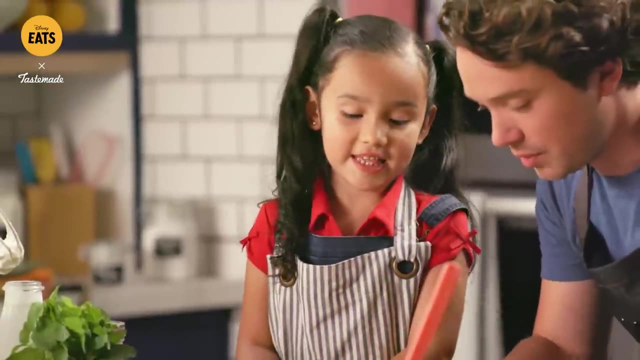 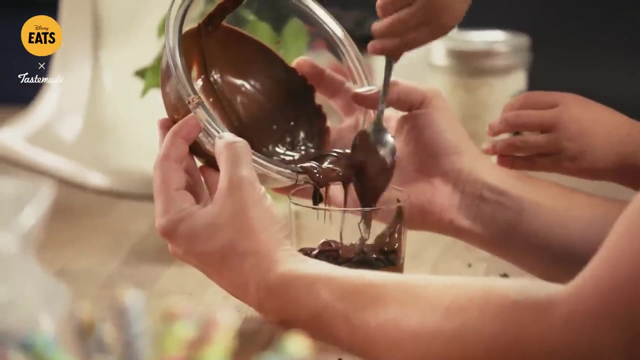 can be neat here. okay, you want to do it, or you want me to do it- me because i got the box. okay, job, all right. all right, all right, that's enough. now more cookies. okay, now we'll put more in. okay, okay, now we'll put more cookies. 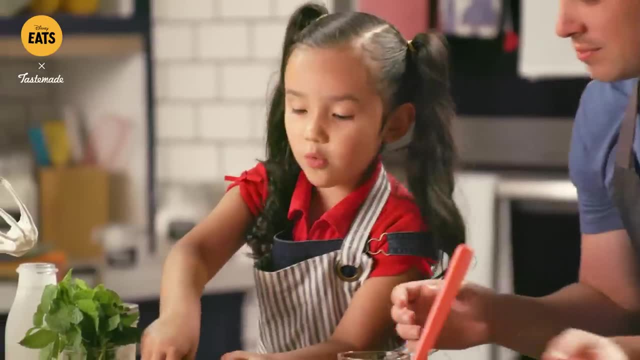 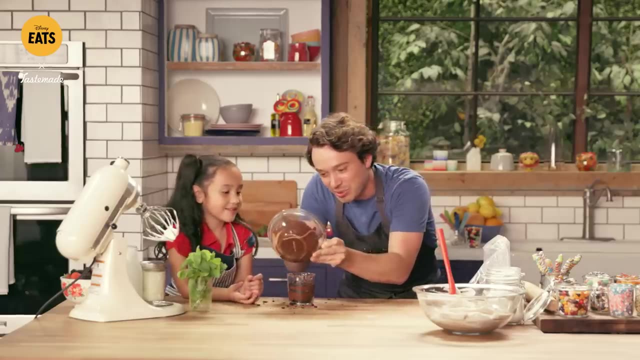 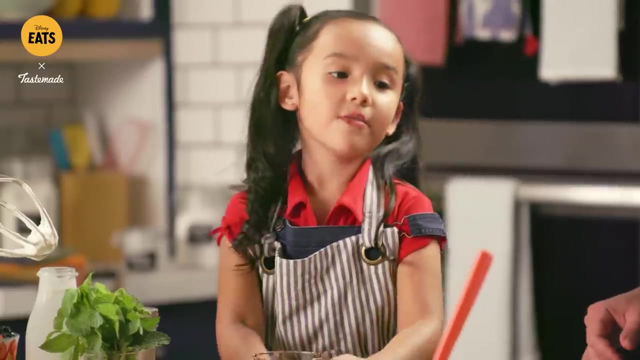 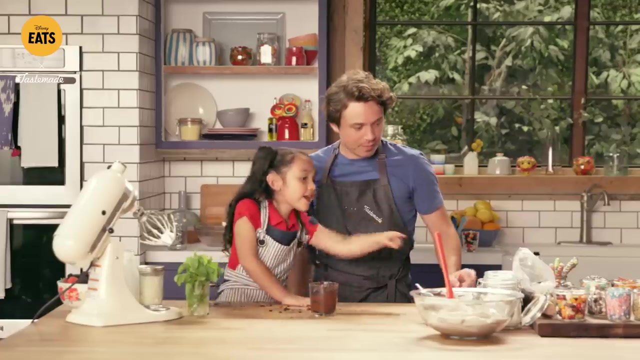 okay, now we'll put just one. one more scoop more. i know, i know i gotta use the side of the spoon so you can get the chocolate. do this fabulously delicious. now one more scoop of cookies. okay, first we're gonna put some candy rocks here. they are like this: yes, so we're putting the rocks on here. done, okay, now we're. 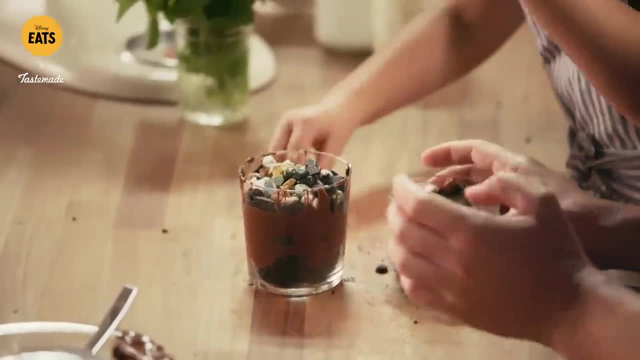 gonna need to stuff the chocolate. so you're doing all these things here. we're going to do the same thing. we're gonna do the same thing here, so you don't have to put it all in at all. you're gonna have to do all the chocolate. you're going to put chocolate in it and then 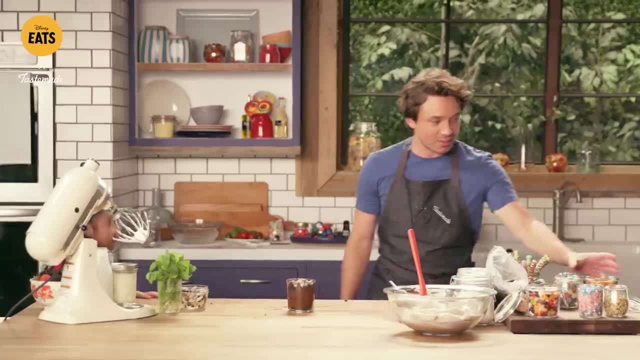 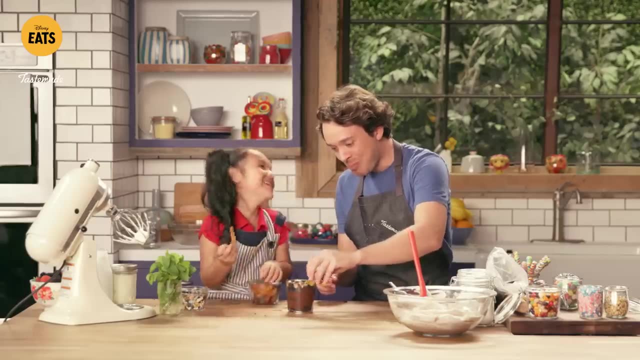 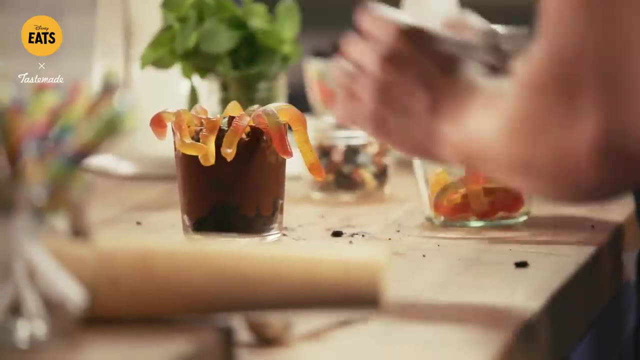 mix them together. so it's all good, now we're gonna use the same spoon and then we're gonna gummy worms. I have those right here. oh great, like this sticking out on the sides there. that's good enough. okay, now we'll need mint. oh really, like a tree, just like that. 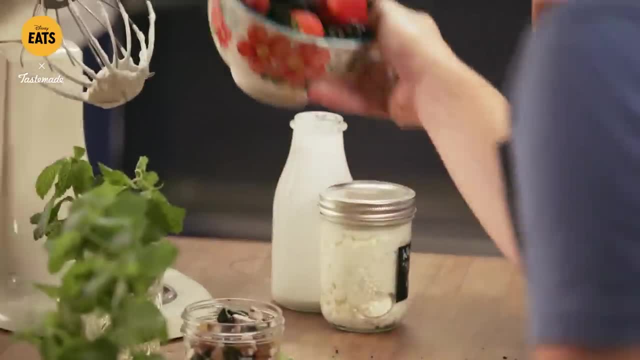 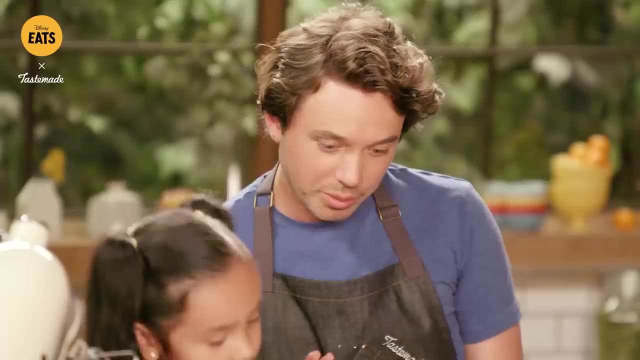 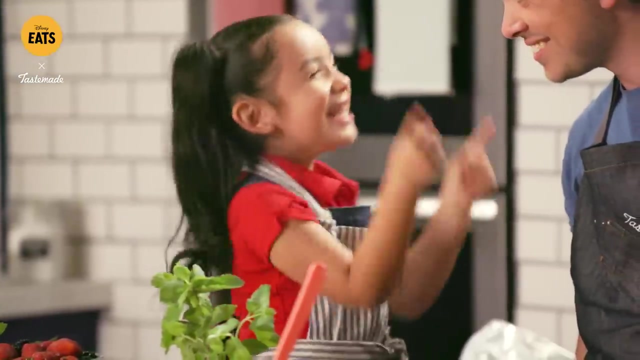 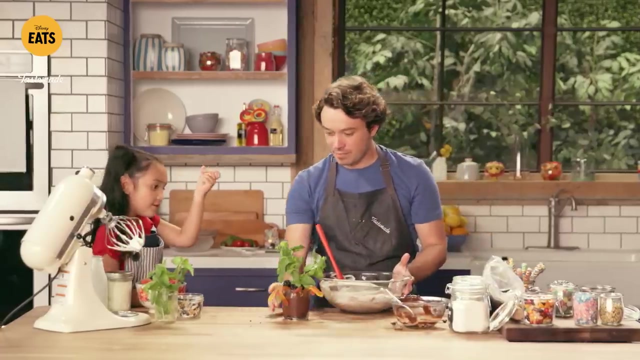 yep, Wow, some berries. so we're putting blackberries all the way around. nope, just a couple. it's really pretty, Sammy. now I think there's one last thing. what about all that whipped cream? that's what I would just, oh great, what are we doing with it? so we're gonna grab it. grab spoon, that's the size. 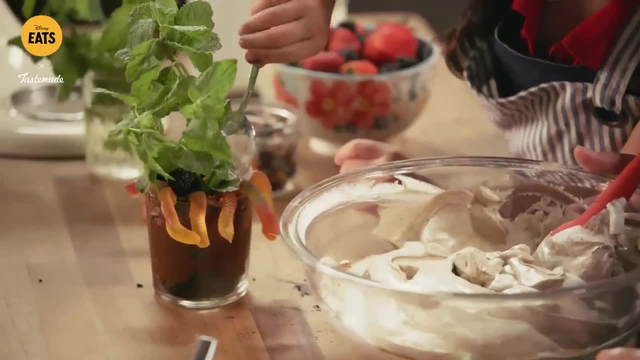 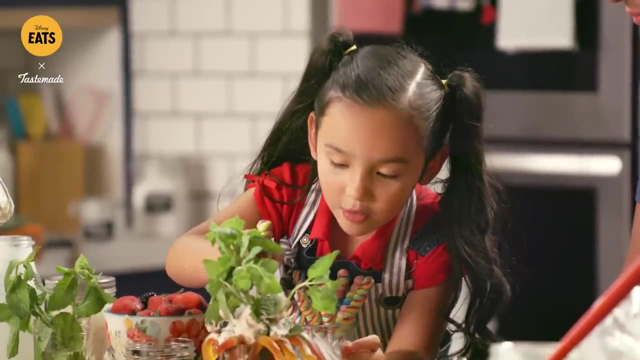 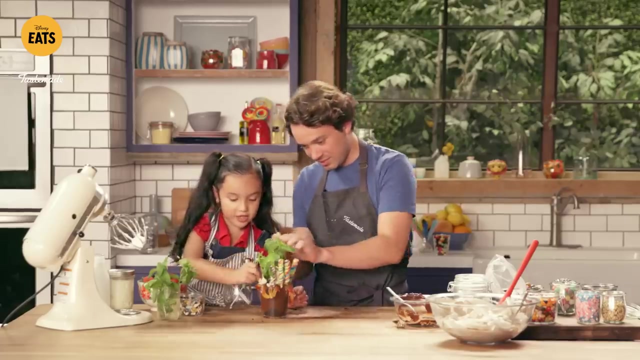 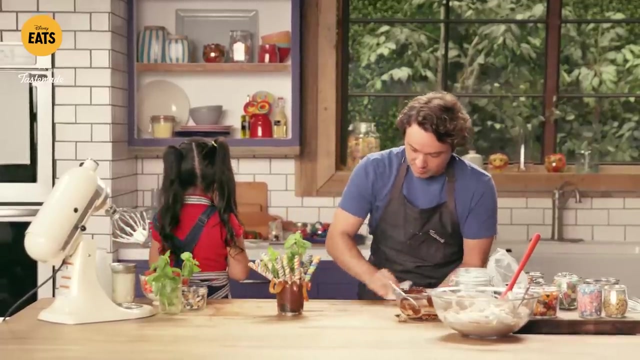 we're gonna take it and put some whipped cream and you're done, okay. one last thing: do you see these little holes? we're gonna stick these in all around, because it will look nice if it's all around. I mean gorgeous, gorgeous. okay, now after that, maybe. 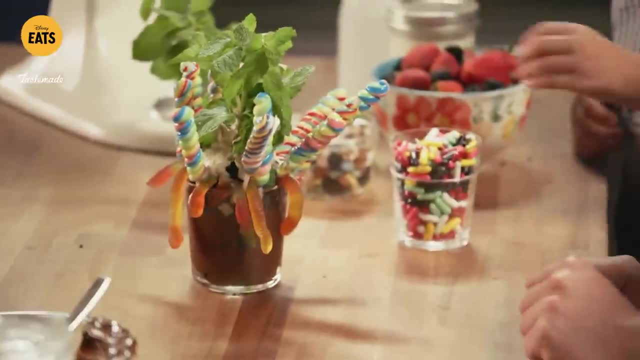 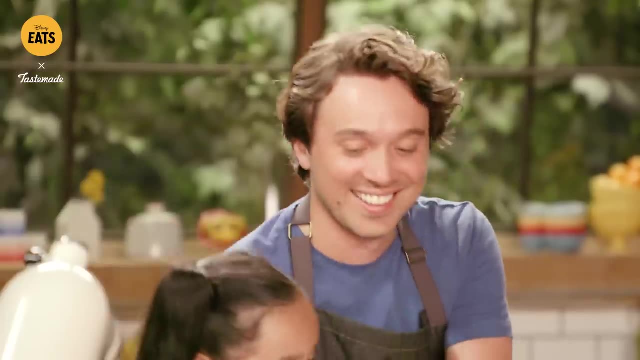 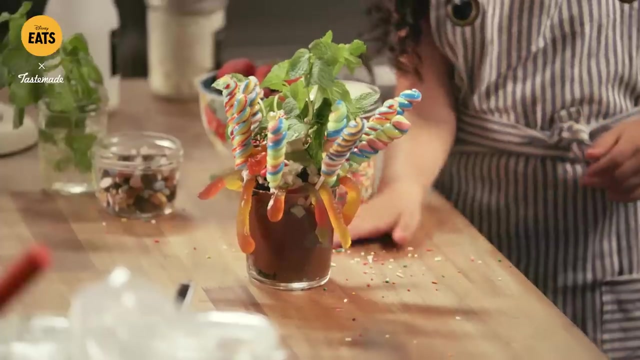 we'll need some of sprinkles. okay, you're gonna sprinkle it from up high down low, put your head in the middle and wiggle it like. so this is very nicely decorated, thank you. that's why I'm the greatest artist- food artist, Frankie. before I tell you what this is, let's clean up this messy mess, no problem. 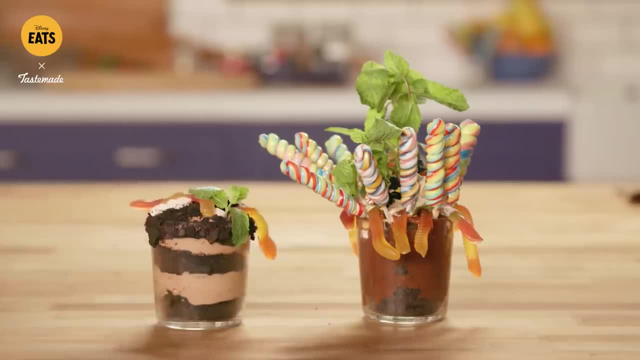 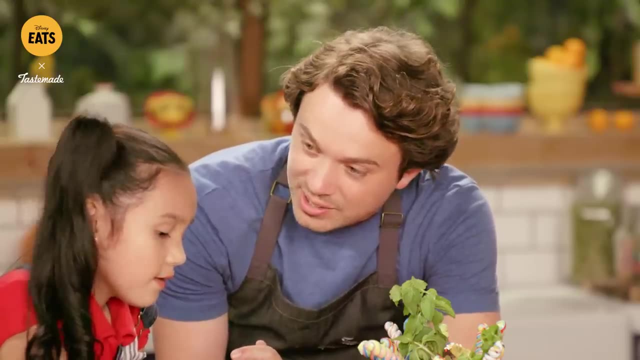 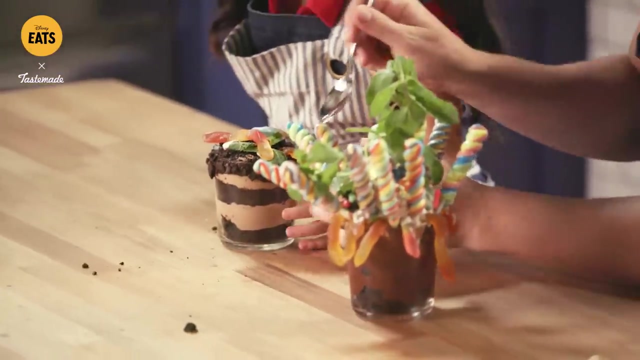 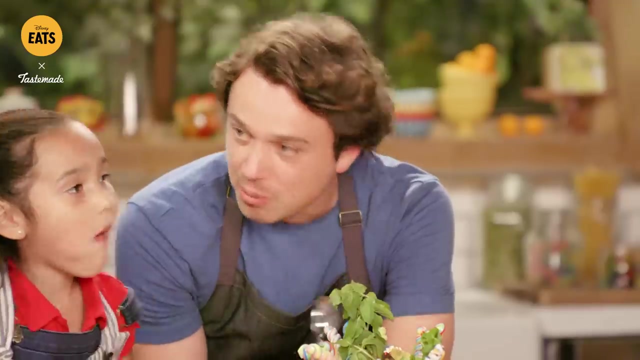 so here's ours, Sammy, and here's the video you watched. what's this one called? do you think Timon and Pumba would like to eat this? yeah, so, Timon and Pumba, you want to try the original one first. so good, you ready to try ours? 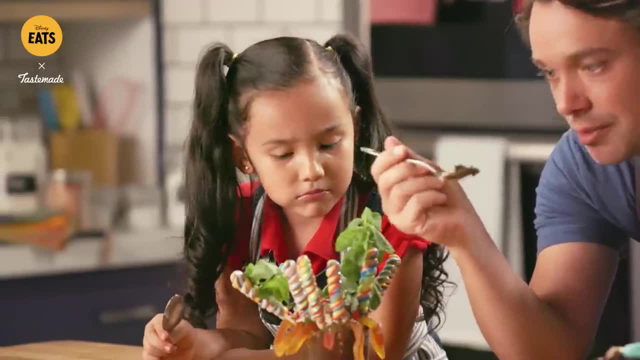 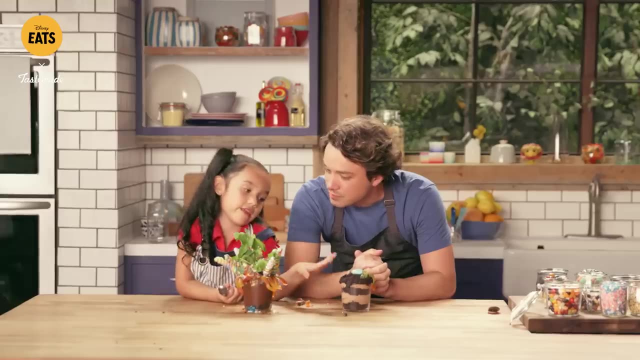 okay. um, it has a lot of baking soda. that's okay. how do you think we did amazing? this is more fancier than this, because you know how of them tell us how. about engaging with a new guy? one of these guys are cool. today we shot so many cool pictures. this is aーレ 欸. 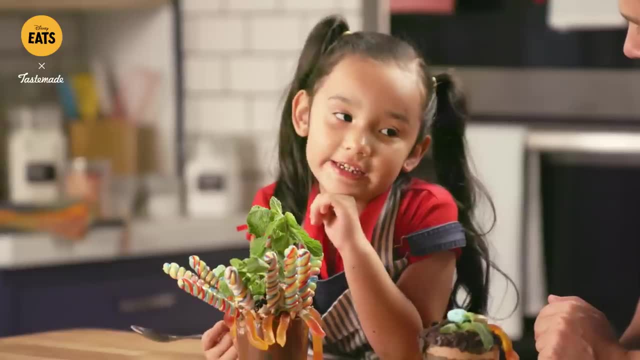 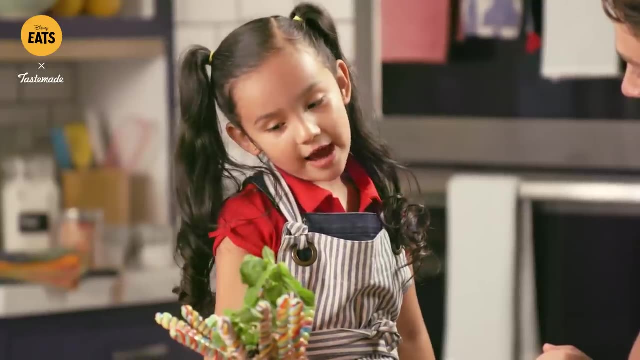 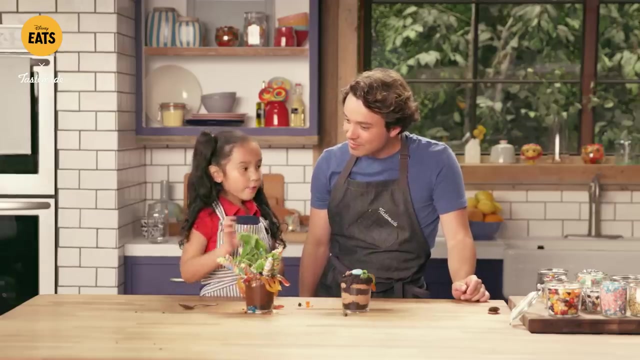 What do you think I did as a cook that was following your directions? Well, Frankie, Yes, The thing is, you kept laughing. I really like your laugh, I kept laughing. I really like my laugh, And I was thinking that you did a great job. 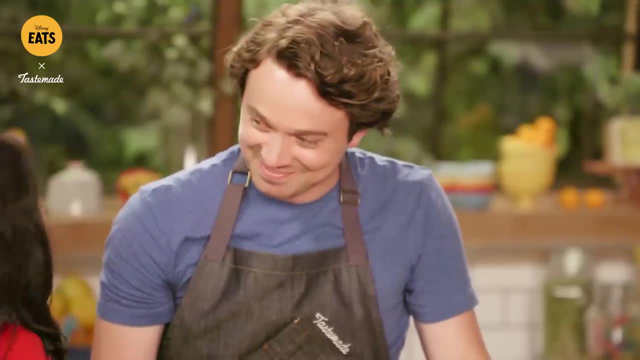 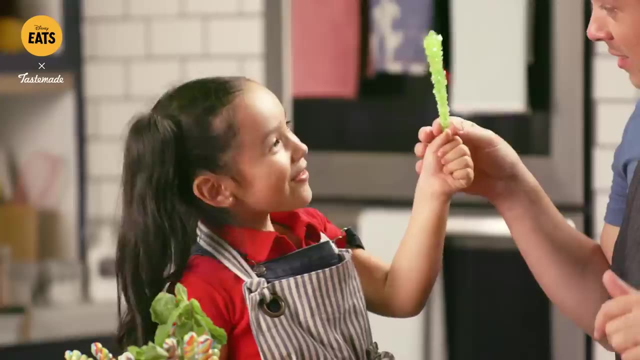 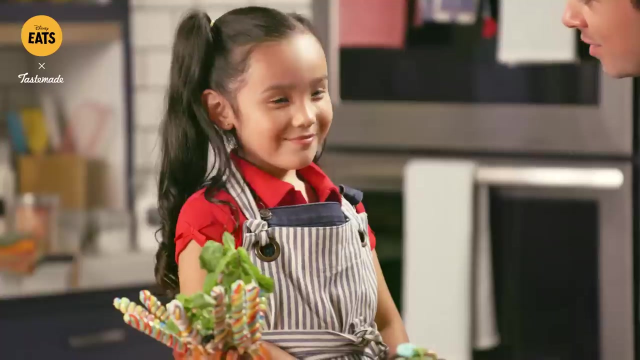 as being a good boy, And I think I'm gonna give you a prize. Close your eyes, Ta-da. Thank you, You're welcome. Well, you know what? I had a lot of fun cooking with you, Sammy, And I think ours is more beautiful than the original too. 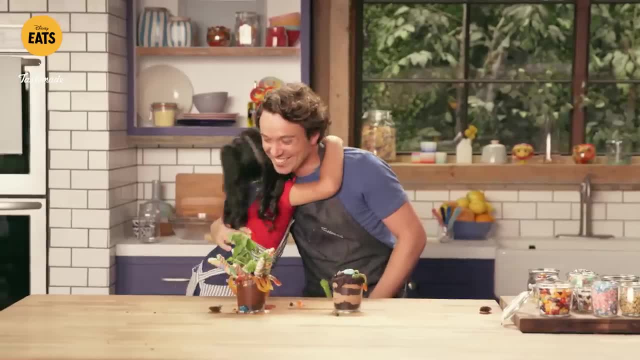 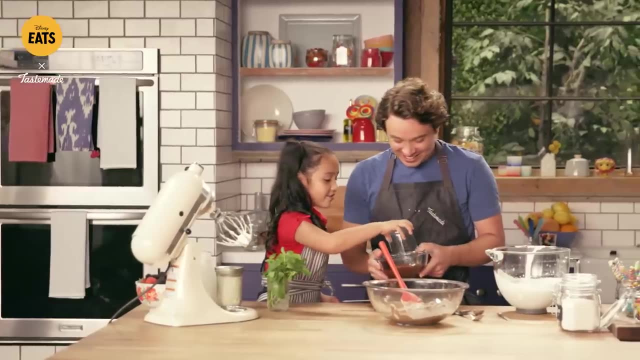 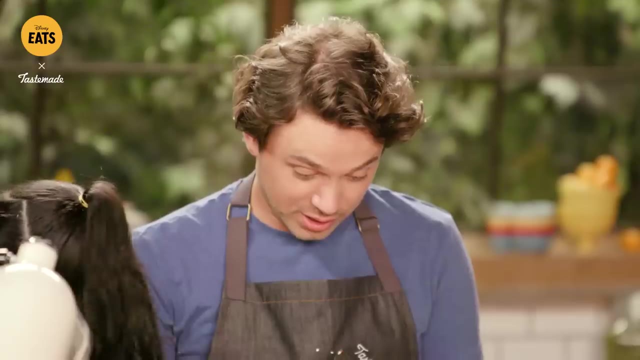 So it's a win. We did it. We did it. Now we do this. Okay, now wash the cup, cause it got a little bit of that, Okay.